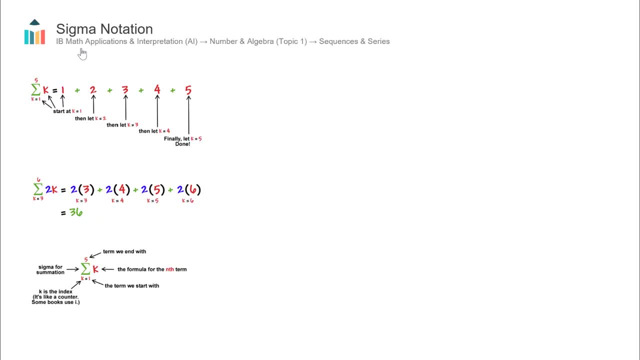 This video covers Sigma Notation, a concept found in IB Maths, AI, in Topic 1, Number and Algebra, which is grouped under the subtopic of Sequences and Series. So so far, in Sequences and Series, you would have covered Arithmetic Sequences and Series, Geometric Sequences and Series. 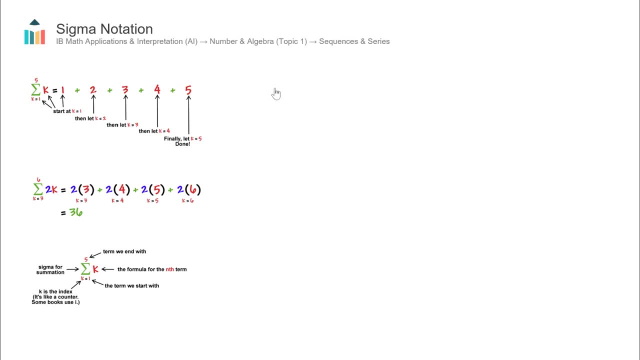 finding Term Values and finding Sum of Term Values. This is another concept added on which is around a different type of notation to show the sum of a certain number of terms in a sequence, and this is called Sigma Notation. Now there are a few examples here on the left-hand. 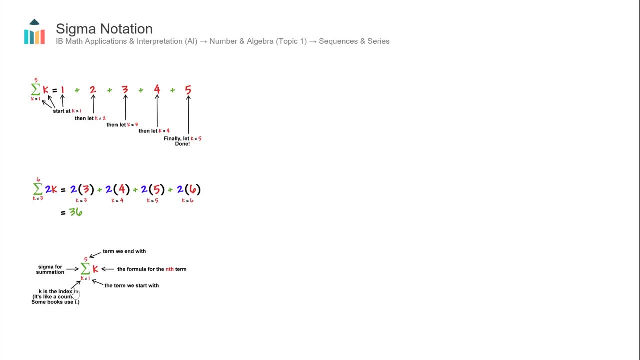 side, both with actual numbers, and then we have the sort of actual notation. Now it looks quite complicated and you may have seen these in maths movies like A Beautiful Mind or Good Will Hunting, potentially written up on maybe a window or a whiteboard, and it looks really complicated. 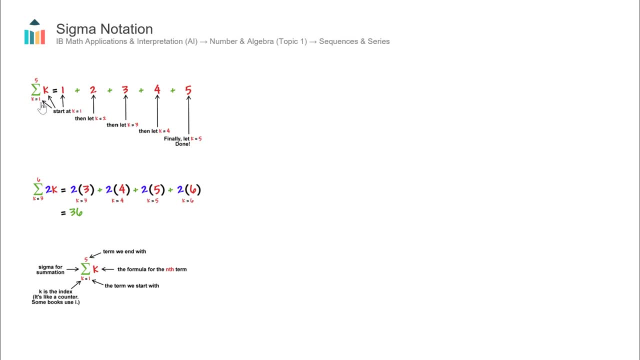 but it's actually not. It's just a concise way of writing out the sum of a certain number of terms in a sequence. So let's talk through an example here. So we have this symbol here. This is a Greek letter called Sigma. It's: 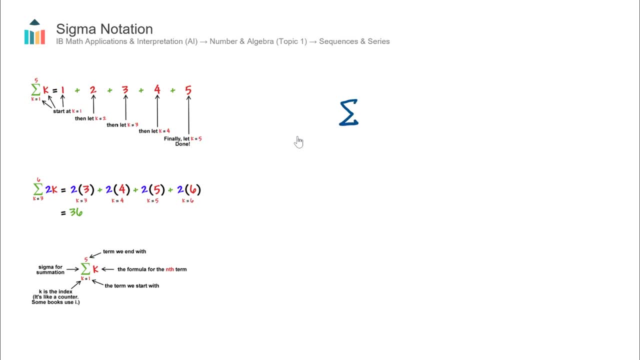 like a big kind of reverse S. Now we have a few different parts to it. This symbol itself actually means sum. Now we have a number on the bottom of the symbol. So this would be, say, K. no, I'll get to why we use K, but K is equal to 1.. Now this is known as our starting point. 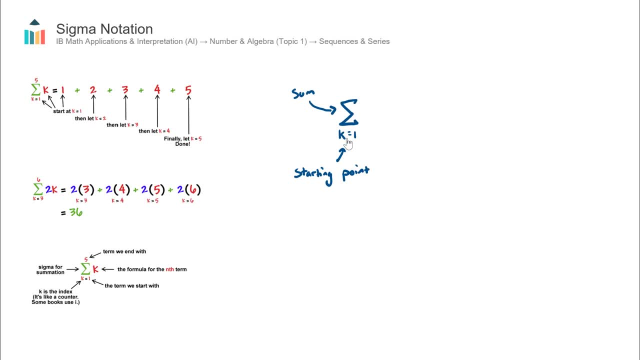 And then we have a number at the top. Let's say it's 4, and this here would be our end point, And let's say our actual formula that we're trying to find out is, let's just say it is K plus 3.. 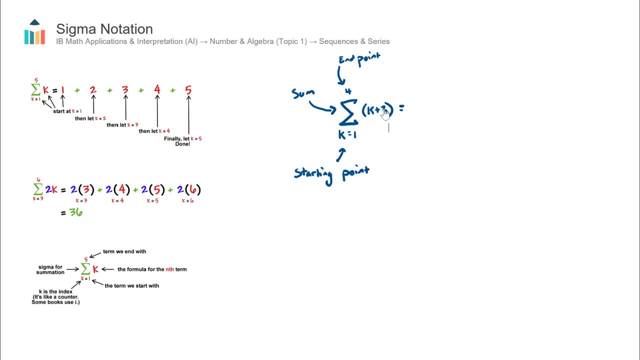 Okay, so what does this mean? Well, we have this formula here: K plus 3.. Now we're going to start at a K value of 1, and we're going to end at a K value of 4.. So let's talk through how we compute this. 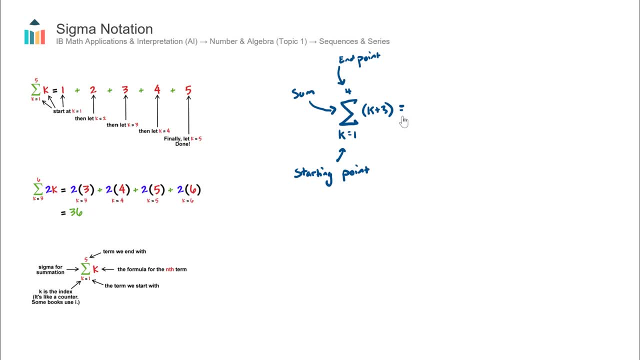 Well, the first term we're going to substitute in, K equals 1.. So it's going to be 1 plus 3.. So this here is when K is equal to 1.. Now again, Sigma means sum, So we're now going to. 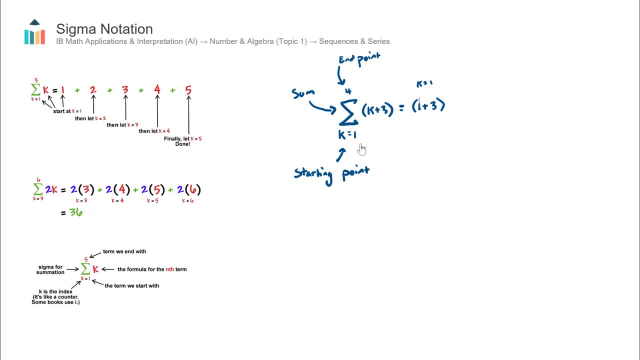 add the next term in the sequence, which will be: so add, and we go up by whole numbers, So it's going to be 2 plus 3.. So this has a K value of 2, plus 3 plus 3.. So that's a K value of 3, plus 4 plus 3.. So that's a K value of 4.. 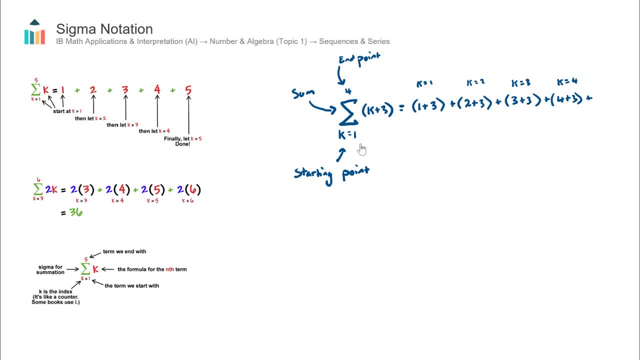 Now do we keep adding? Do we go again? Do we go to K equals 5?? Well, we don't, because we know it has an end point when K is equal to 4.. So we actually end at this point here And we can find out what that is. That is 4 plus. 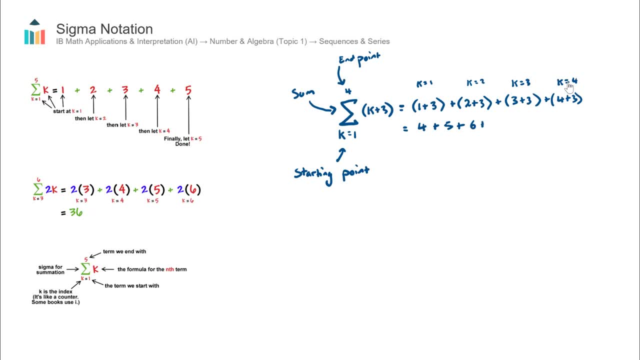 and this one here is 5, plus 6 plus 7, and that is equal to 9, 15,, 22.. So you can see here this: although it looks complicated, there's just a concise way to say. 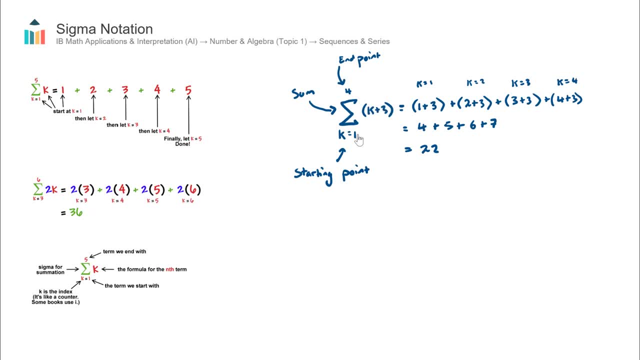 hey, we have K plus 3 here as my formula. I want to start at 3 and end at 4 and sum all of the terms up, And that's just sort of how it plays out there And it gets to finally the end point. So we can find out what that is. So we can find out what that is. 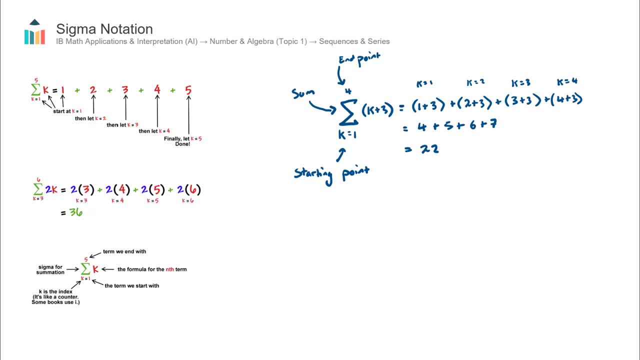 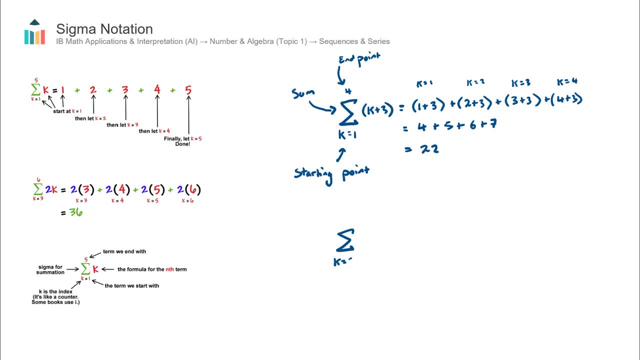 meaning sum. Let's go from a starting point of K is equal to 3.. Let's end it at 6.. And my formula here is 1 on, let's say, 3 to the power of K. Okay, so the first term will be 1 on 3 to the power. 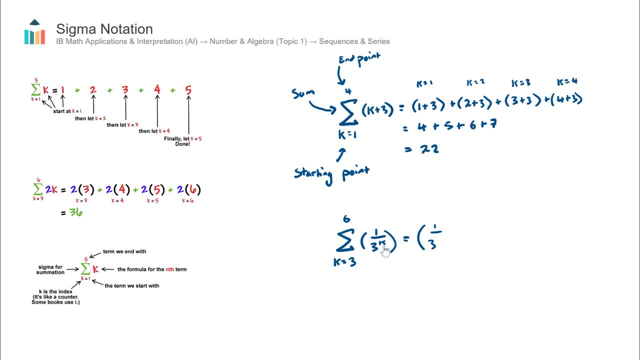 of So 1 on 3 to the power of Now. it's not going to be to the power of 1 this time, because I'm actually starting at 3, so it's going to be 1 on 3 to the power of 3. so this is a k value.